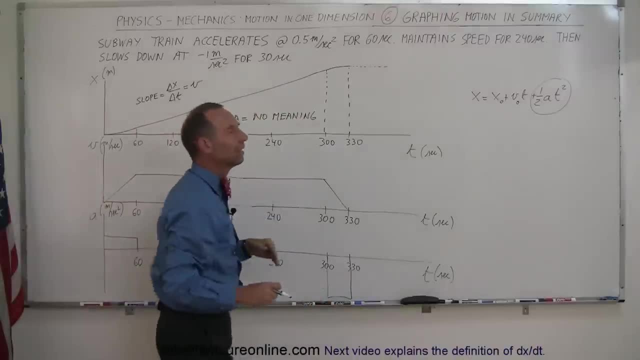 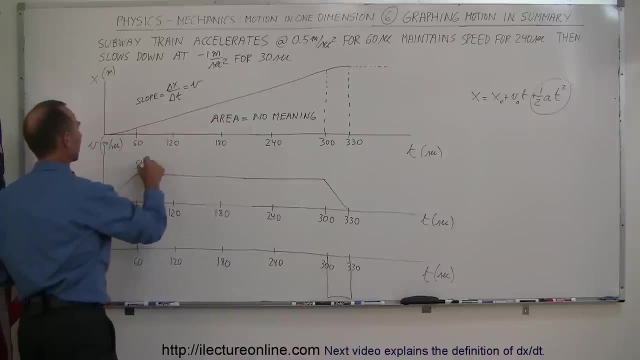 That means velocity is constant. Here the slope is decreasing. Velocity changes back to zero. On the second curve we have velocity versus time. The slope here represents the change in velocity over time, which by definition is acceleration. So here you can see: you have a positive slope, positive acceleration, zero slope, no acceleration. 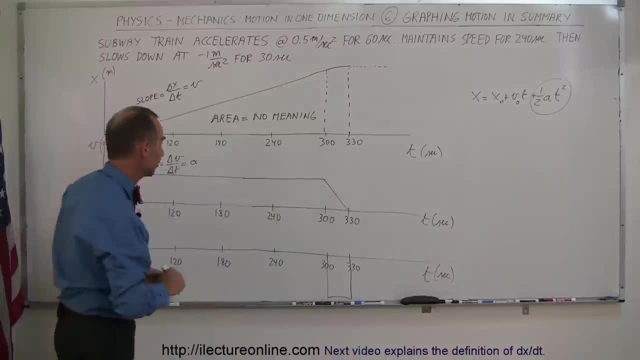 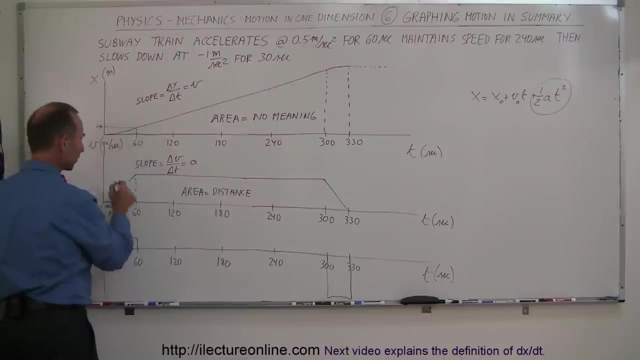 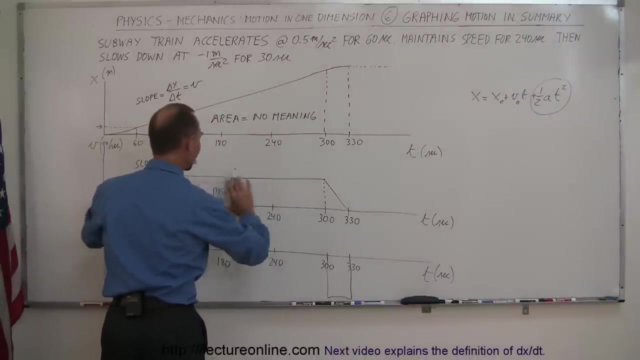 Negative slope, negative acceleration. The area underneath the curve represents distance traveled. Notice, the area underneath here represents the distance traveled in the first 60 seconds. So this quantity right there is determined by the area in this rectangle. Then the area traveled during the 240 seconds where the speed doesn't change that rectangle right here, the 240 seconds times 30 meters per second represents the change in velocity. 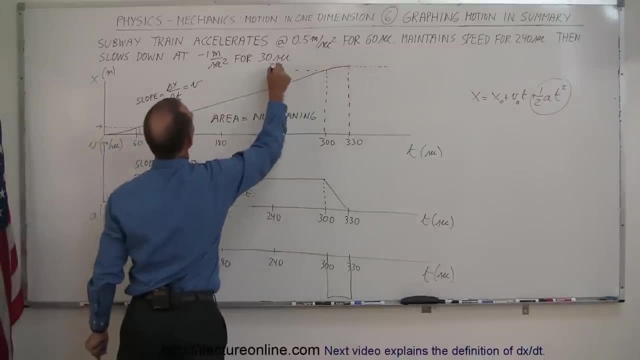 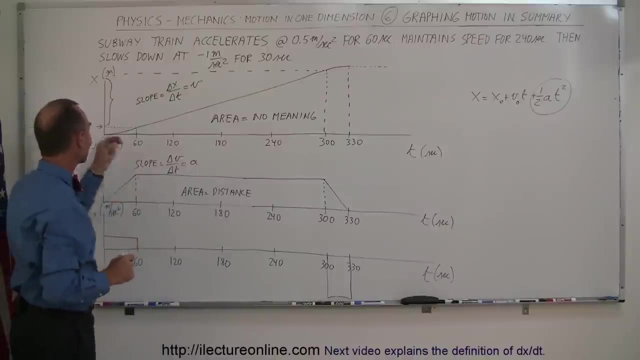 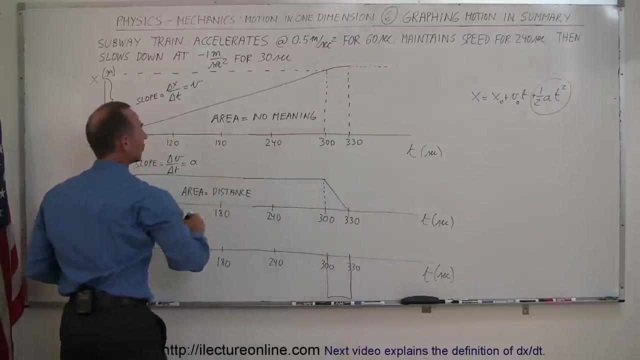 The area here represents the distance traveled during the this time period. So that represents this distance right here. So we add the first area plus the second area and we get up to this number right there. And then, finally, this area right here represents the distance traveled while it's slowing down. 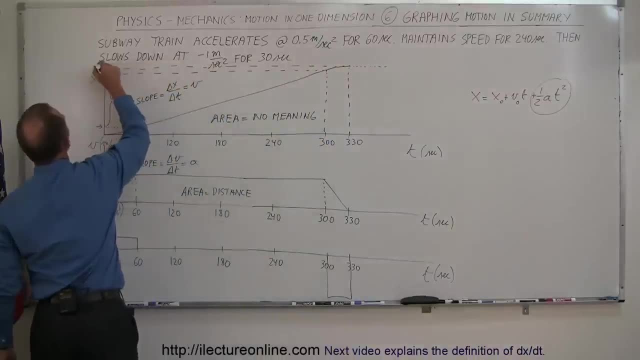 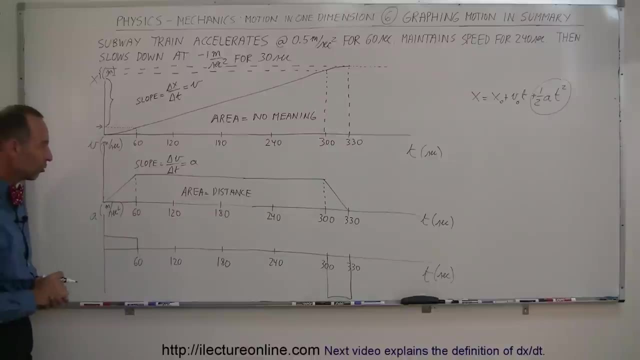 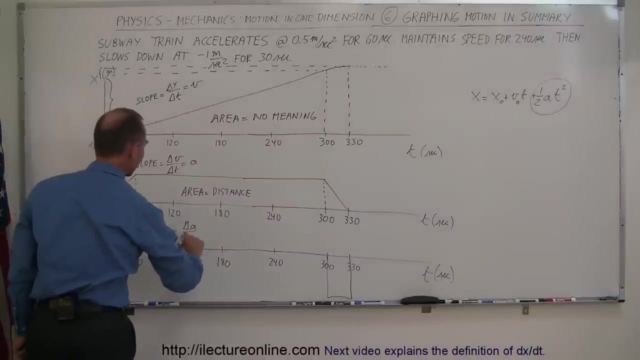 And so we can see that if we take this curve over here, this distance right here or this amount right here represents the area of that curve right there. So there you see the relationship. Finally, acceleration versus time. The slope represents the change in acceleration over time, which is simply the derivative of acceleration. how fast acceleration changes. 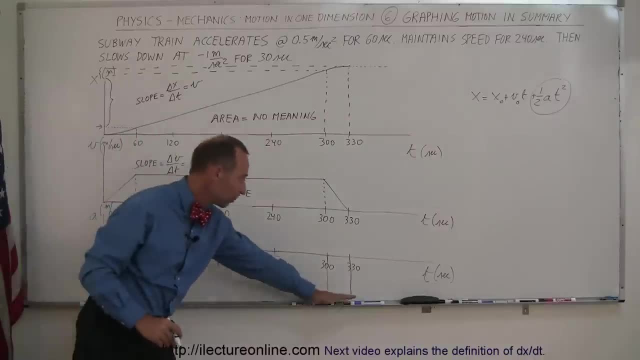 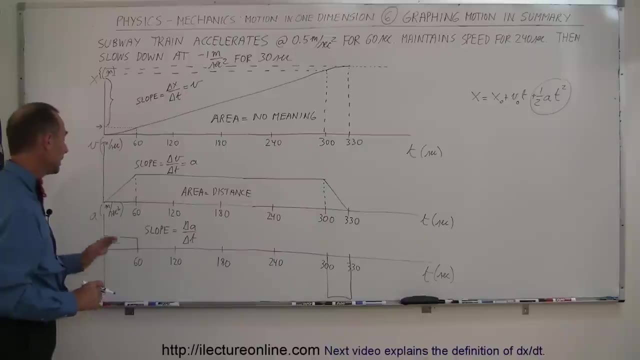 Notice that the slope here is zero. the slope is zero. the slope is zero here, meaning the acceleration doesn't change. It's constant in those three instances. All right, The area underneath the curve represents the velocity traveled. So as time goes by and there's more and more area underneath the curve, 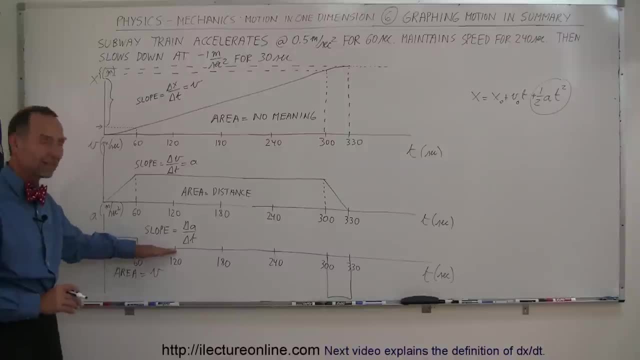 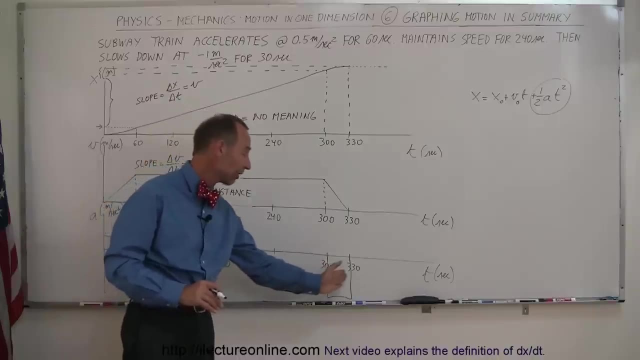 you're going faster and faster and faster. Now you can see there's no more area right there. That means the velocity is not changing. Here the area is negative. That means the velocity is decreasing. You're losing velocity by the time you get back to this point. 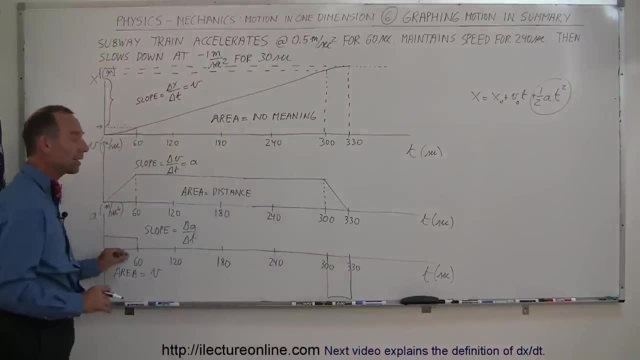 This negative area cancels out this positive area right here and the velocity is back to zero. So the area represents velocity, The slope represents the change in acceleration over time for an acceleration versus time graph. And that's what the graphs look like: X versus t.